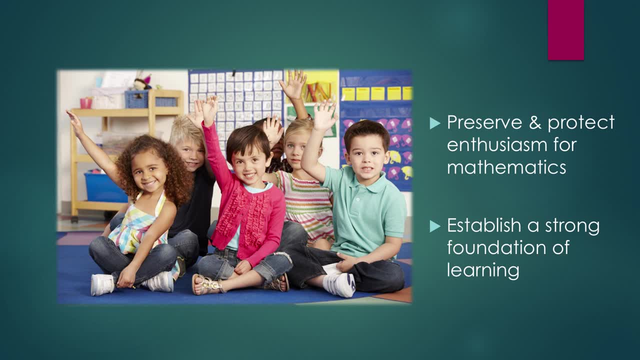 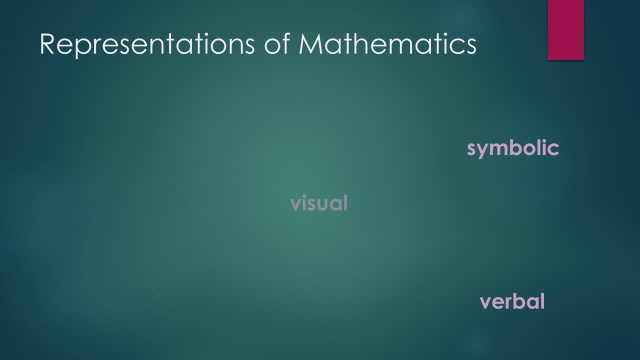 they have for mathematics, They come loving it and by the time they get to middle school, hmm, not so much. We want to establish a strong foundation, we want to keep them moving. so we use all the different representations that we have. What I want to think a few minutes. 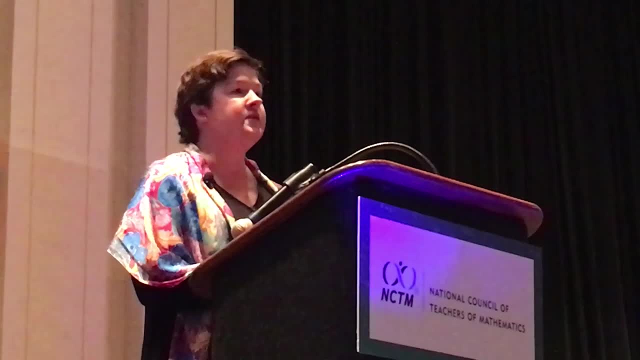 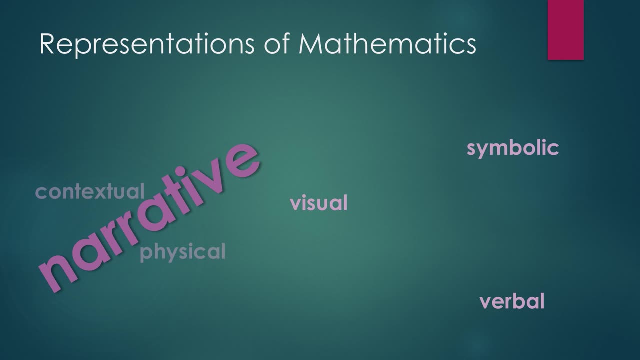 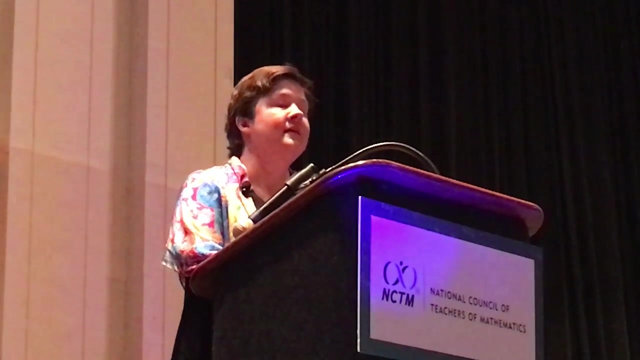 about tonight is this idea that if we bring together the physical representation with the contextual representation, we end up with narrative, we end up with mathematics as story and the story is the math. This isn't read a story, then we do math This. 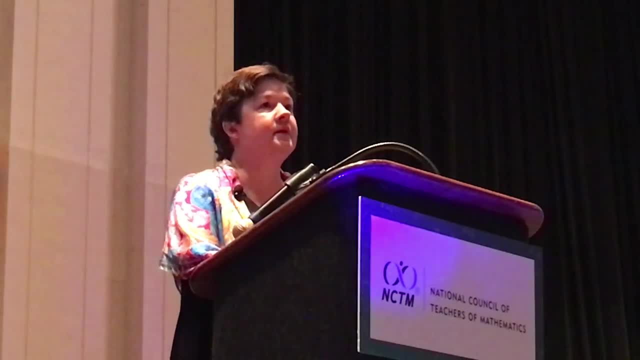 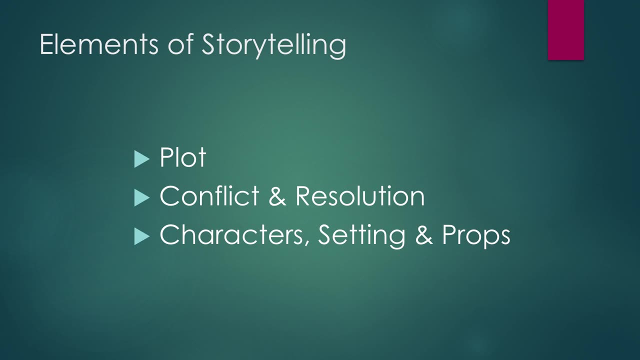 is that the story is the math, It's where it's grounded, And that means that we have to think about, as we work, the elements of story. We need plot. What's going to happen here? We have conflict in resolution, we have characters, we have settings, we have props. 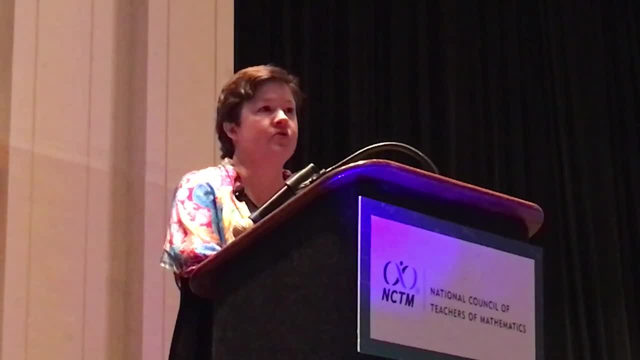 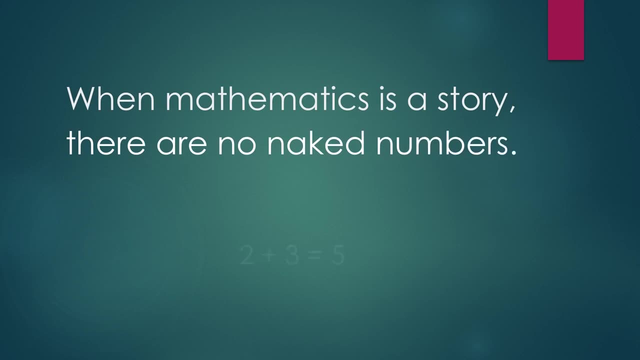 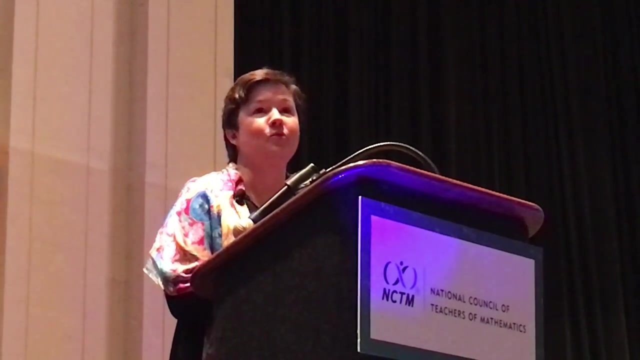 Plots are critical because they're what make the story. mathematical stories, not just a tale. we tell No naked numbers. They really don't make sense, so let's just skip them. It really is one of the most powerful things I think we can think about Our storylines. 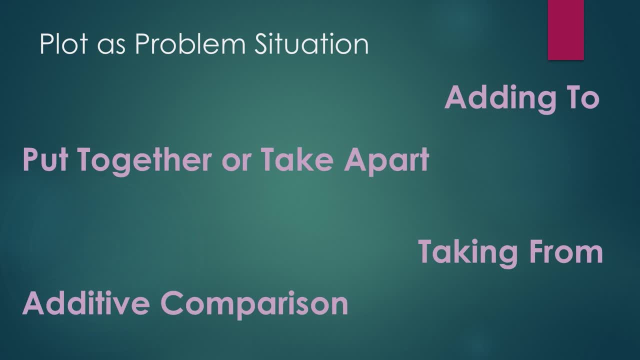 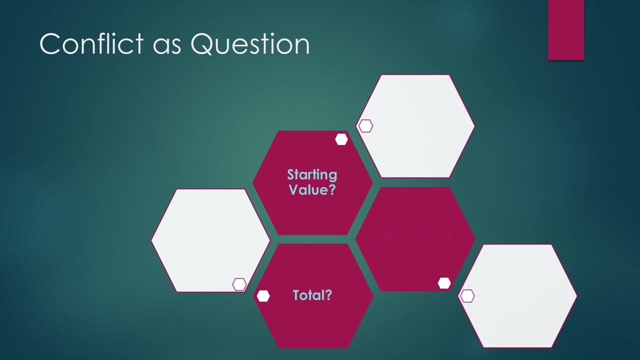 with primary children are really about adding and subtracting. So, if you know table one, these are the four rows and they form the basic plot lines, the mathematical stories that we tell. the conflicts in the story are the questions. what are we trying to figure out? do we want to know what the 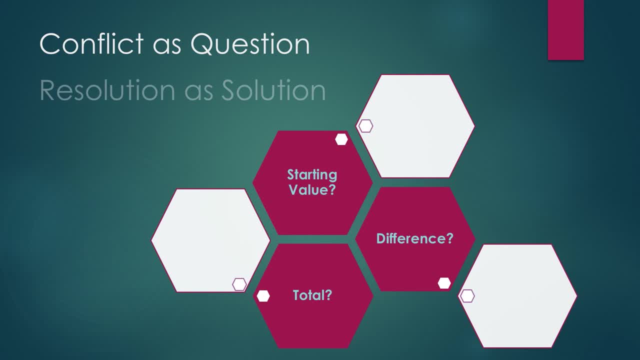 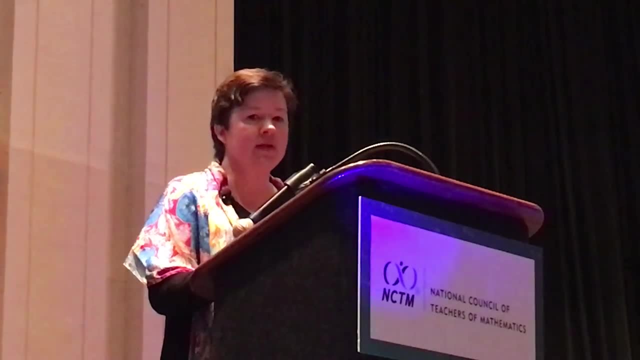 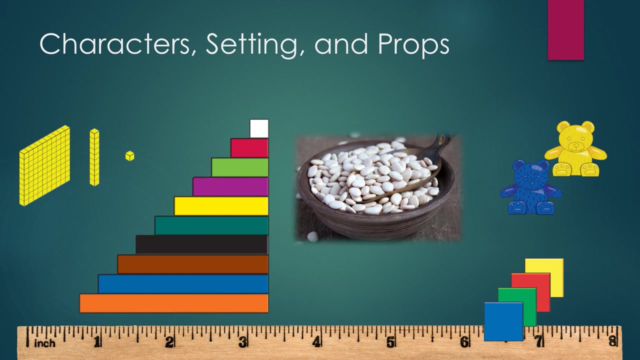 difference is: do we want to know a total? the resolution to the story is the solution to the problem. what's our answer? we're still doing our math, but we're doing it in the context of story, and our mathematical props, whether formal manipulatives or more informal tools, are things that we can use to 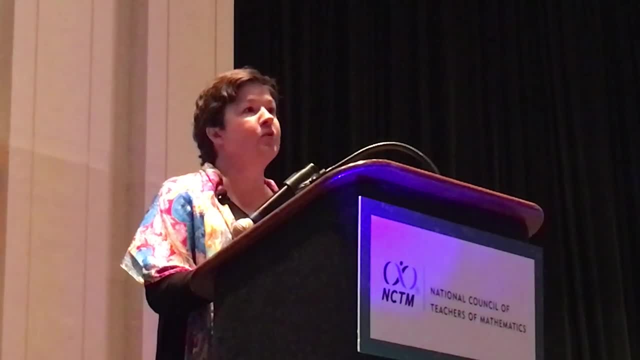 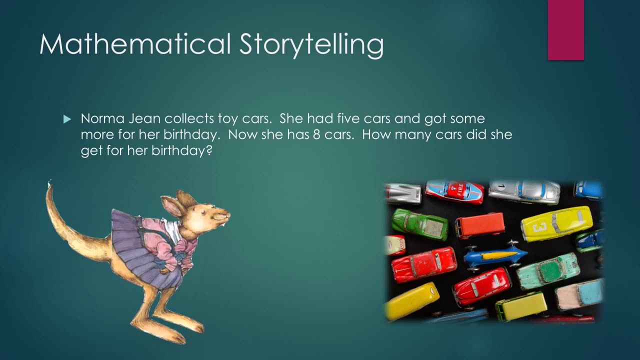 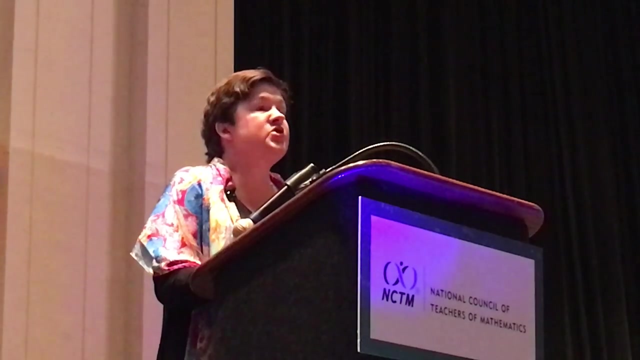 feature and highlight the mathematics. so let me tell you a couple of quick stories about my friend Norma Jean. she's a kangaroo, she likes to jump, she collects toy cars and she had five and then, when she got some more for her birthday, now she has eight and the question is: what's the storyline? what's? 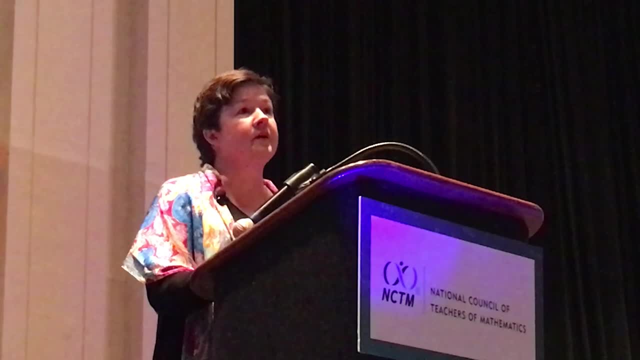 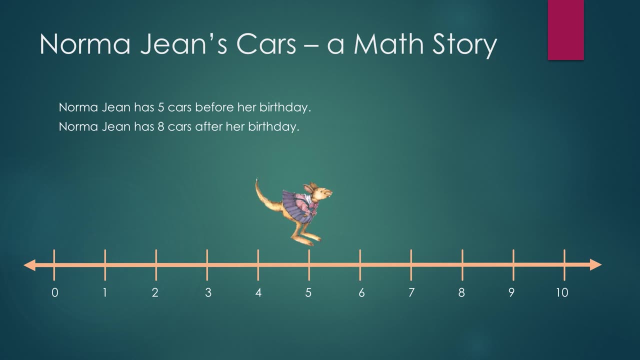 the narrative for figuring out how many she got for her birthday. in a classroom we have a number line in the front of the room and kids hopping along. you get animated. Norma Jean instead had five. how many more is it going to take to be eight? how many hops does that require to? 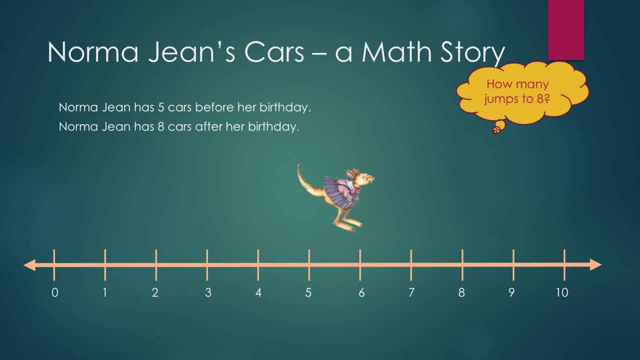 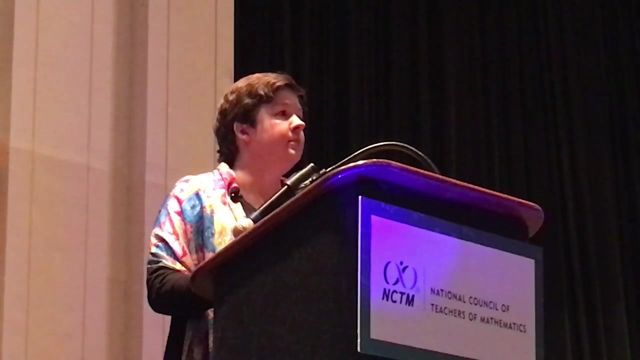 move from five, where I started, to eight, where I am. when children do this- and they are the story, and this story is the mathematics- it brings great power to what they remember and what they learn. is the number line always the right prop? no, is jumping along the number line or a motion at all always the right strategy? 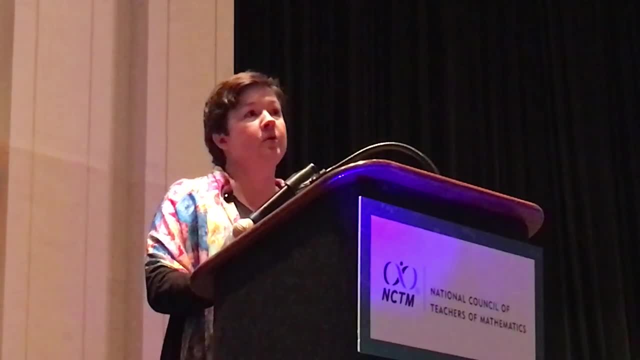 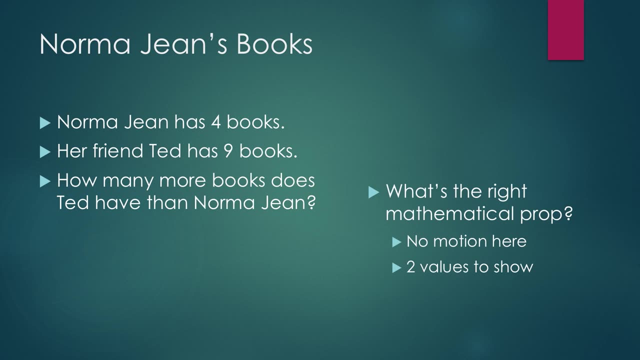 no, depends on the problem. so if we think about Norma Jean and her friend Ted in a different problem, now we're looking at the books that they have. Norma Jean has four, Ted has nine. I don't need a prop that will let me show motion here, but 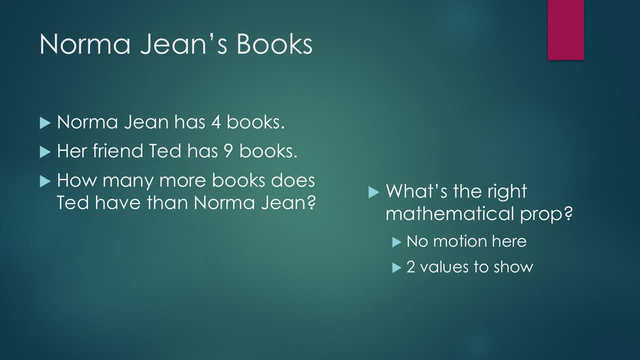 seeing those two values is a really big deal in this work, so I want to choose a model that will let me do that. in this case, I'm going to pick Cuisenaire rod. so my purple rod is Norma Jean's, for my blue rod is Ted's nine. 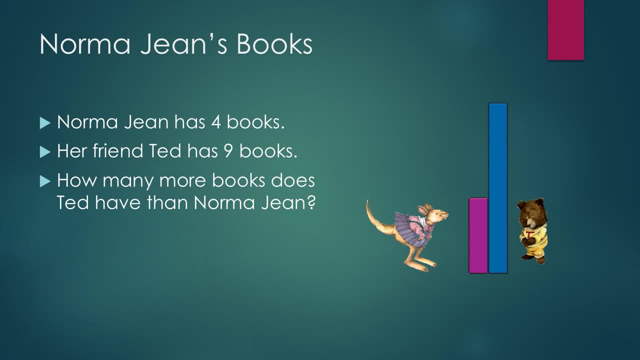 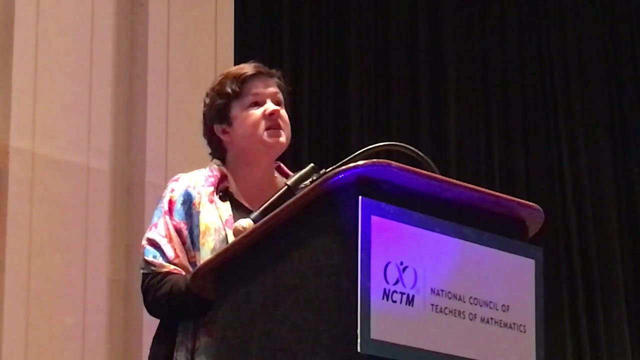 my mathematical question, my resolution to the story. what fills in the gap? What's the piece that comes in the middle and shows us that in fact, Ted has five more books? It's that yellow rod. Could I use the number line as my prop? Sure, That would work, but it's going to look different than 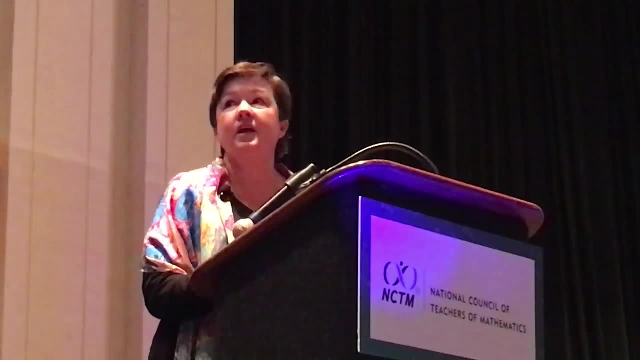 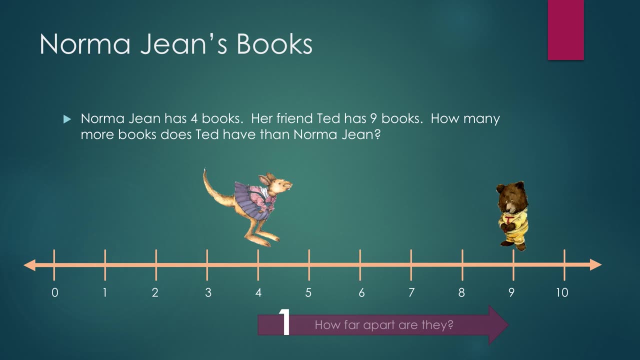 the number line did last time, because I don't need to move here. Nothing came, nothing left. I'm worried about how far apart Norma Jean and Ted are. So in class we've got three kids now. We've got Norma Jean, we've got Ted. we've got a counter to help us think about how that works. 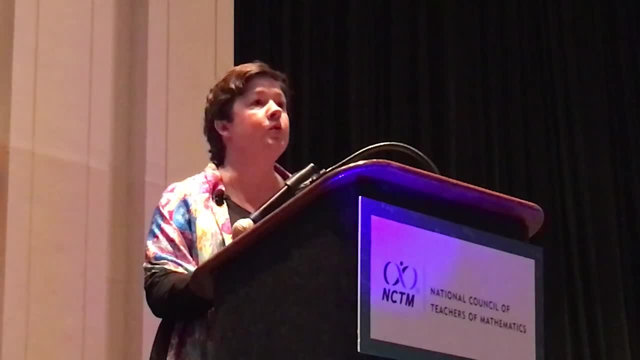 What that means is that we're using these tools, we're using these manipulatives as props. we're thinking about what's the mathematics that they show. how does it bring that to light so that the story is the math for the kids? 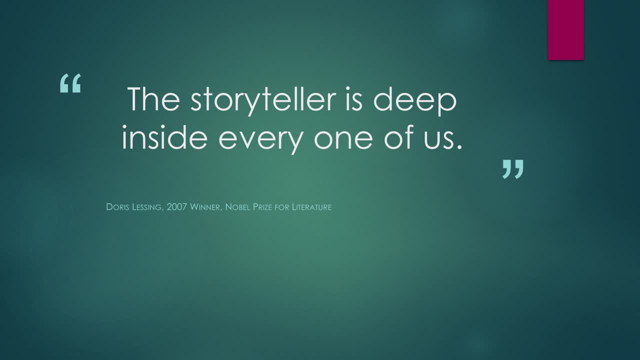 The storytellers deep inside all of us as grown-ups. it's not so deep in the imagination In all of us. It's not so deep in the imagination If we can- supposedly the kids. So if we can dig it out of ourselves and use that as a way of